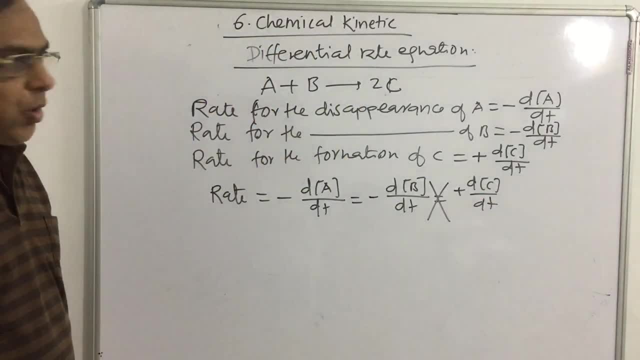 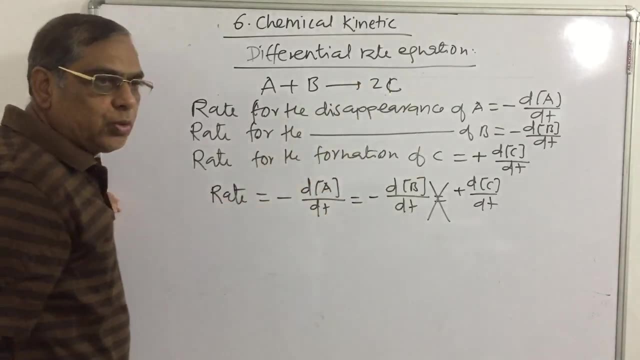 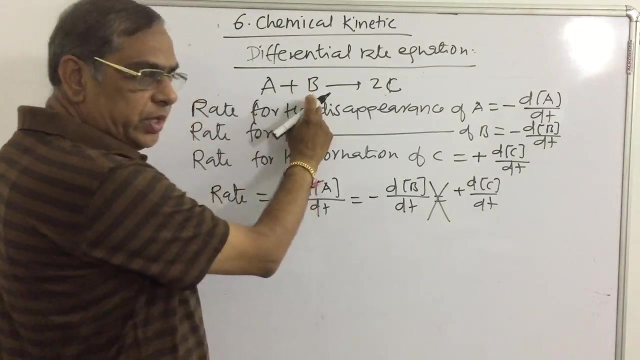 But this equation is not true, Because here, when one more of A combined with one more of B, Then there is the formation of a, two moles of a- C. So when one more of A disappear, one more of B disappear, then the two moles of a C form. 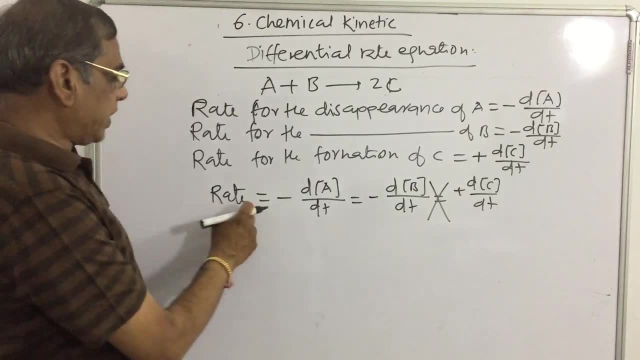 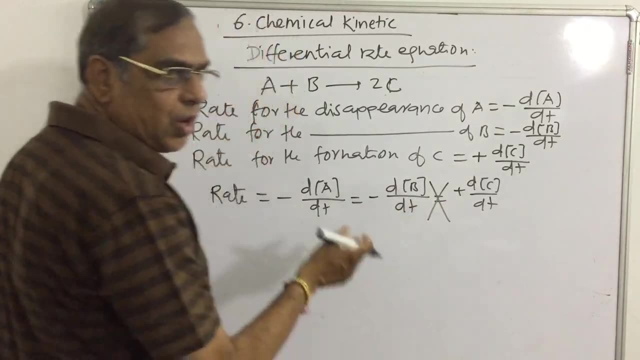 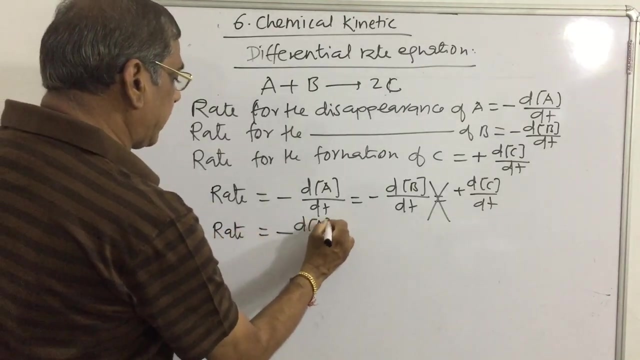 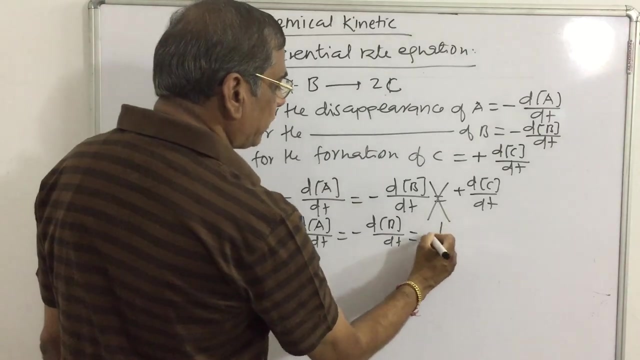 So when we want to determine the average rate of reaction after instantaneous rate of reaction, this equation is incorrect. So in order to determine the correct rate of reaction, We divide the stoichiometric coefficient like that D of B, here divided, that is the stoichiometric coefficient that is 2.. 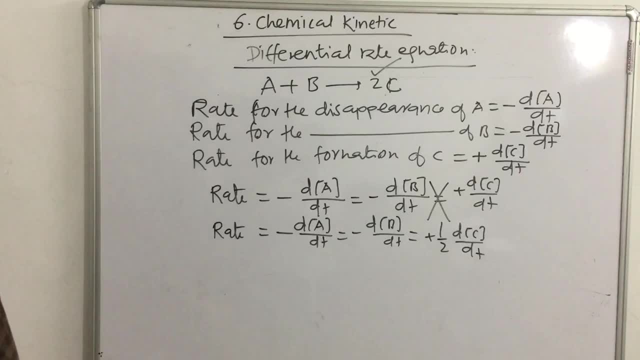 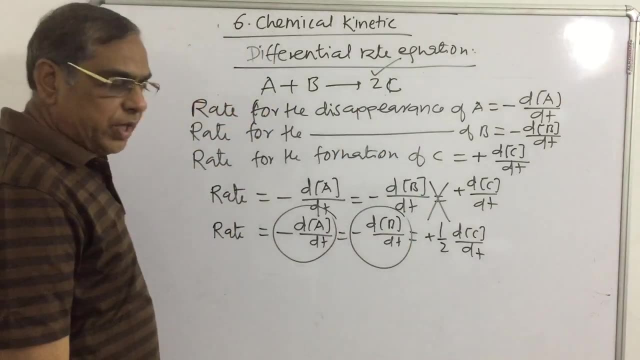 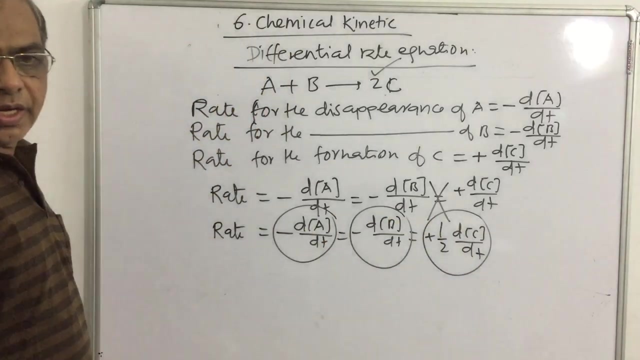 And now this: all are equilibrium. So by knowing the decrease in the concentration of A, or decrease in the concentration of B, Or increase in the concentration of A, Or decrease in the concentration of C, divided by 2., You can determine the rate of reaction. 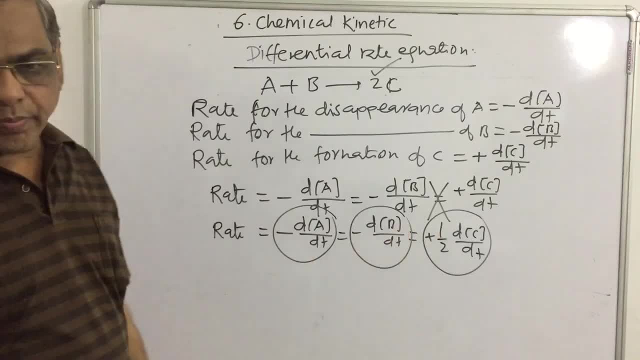 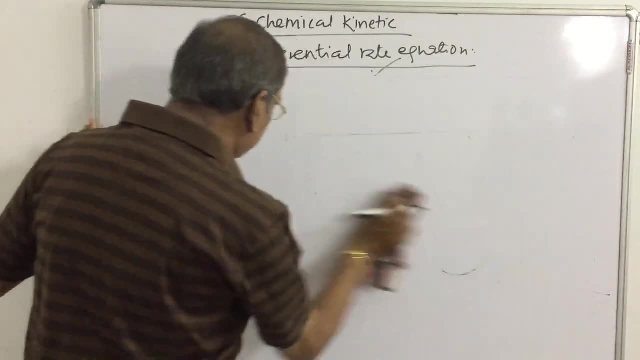 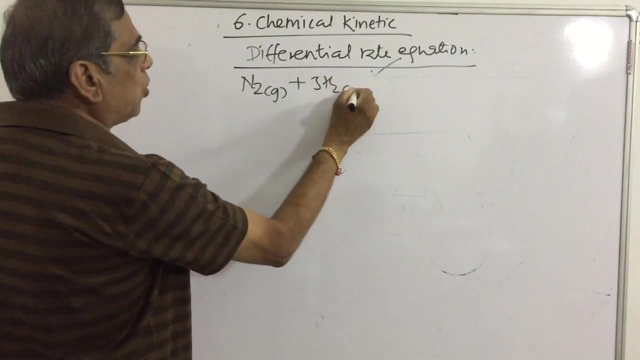 Now all these terms are in equilibrium. Again, we consider the next example, that is, the formation of a ammonia. For a formation of ammonia, that is, the nitrogen gas combined with 3 moles of a hydrogen gas, formation of 2 moles of a ammonia gas. 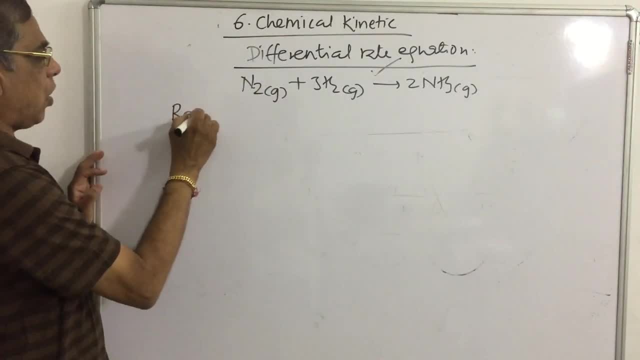 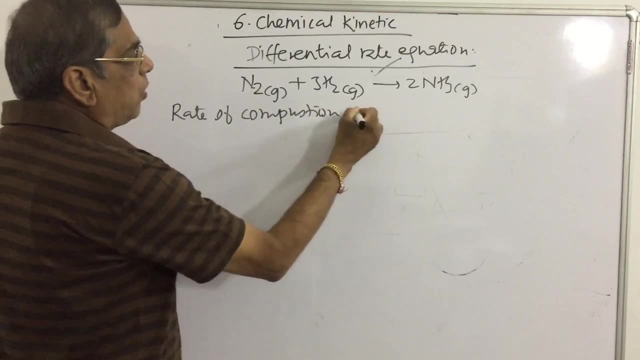 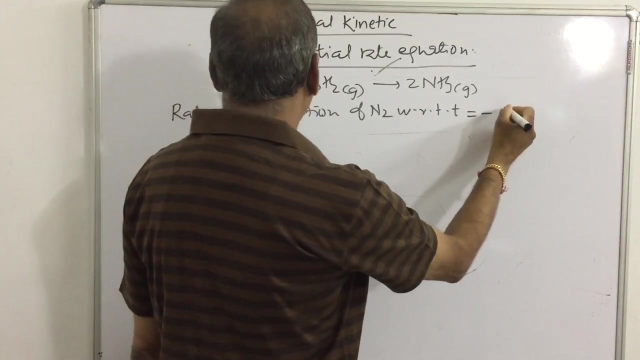 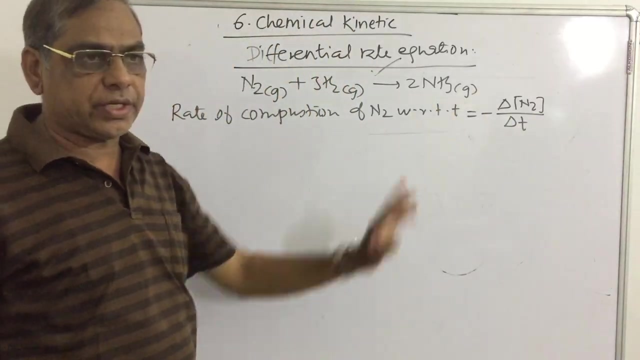 Now here, what is the reaction? What is the reaction? The rate of consumption of nitrogen with respect to time. We can write: that is the minus change in concentration of a nitrogen with respect to time. Here average rate is taken, So capital delta is taken. 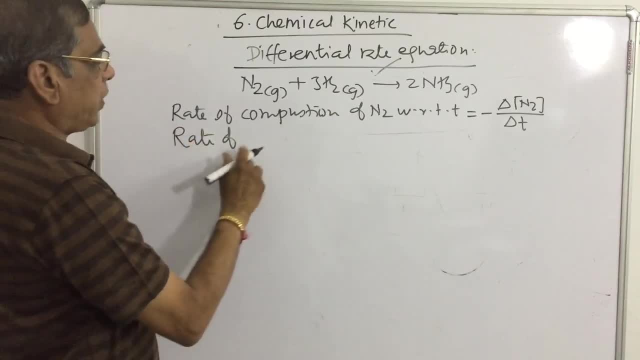 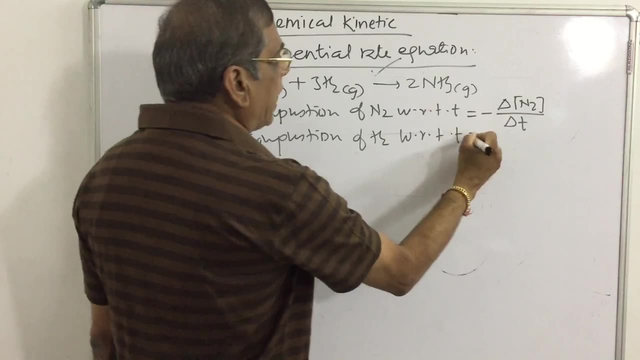 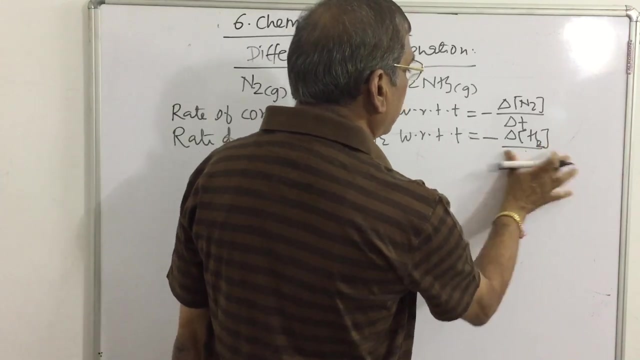 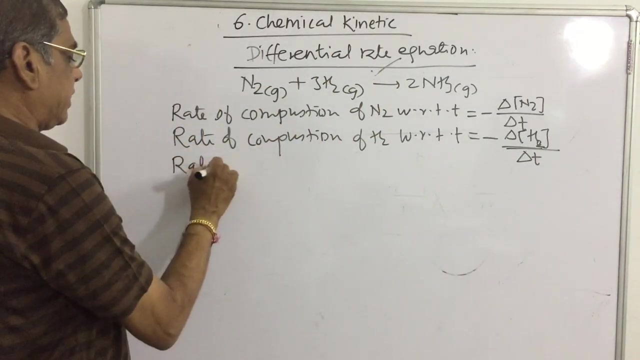 Suppose again the average rate of consumption. Consumption of hydrogen with respect to time, That is the decrease in the concentration of a hydrogen with respect to time. Decrease in the concentration of hydrogen with respect to time: Here, that is the rate of formation of ammonia.